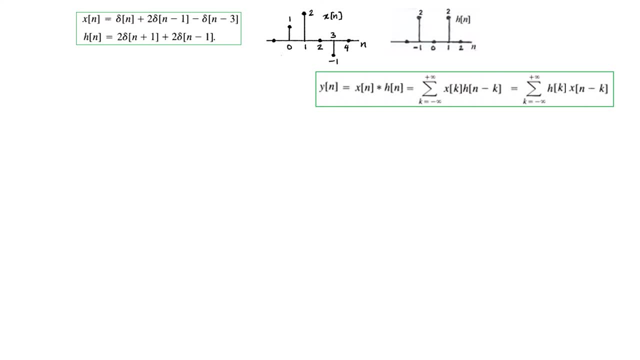 the idea n equal to 0, so we start at 0. and Delta means amplitude 1, so we draw amplitude 1 signal here. This one is n minus 1, when we put n minus 1 equal to 0, that means n. 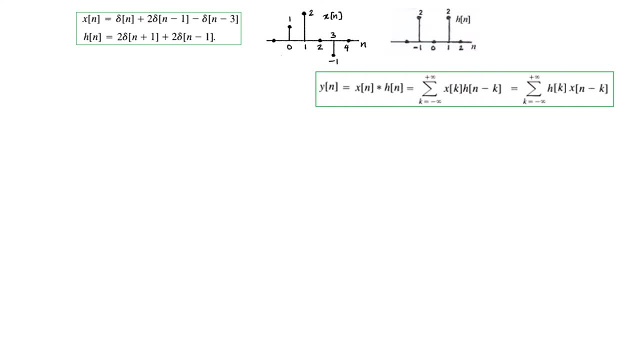 is equal to 1.. 다시 해�dio. we are at point. n is equal to 1 and we have 2 delta. that means the amplitude will be double. so in this way this is plotted, and same way the hn function is also plotted. we have 2 delta. 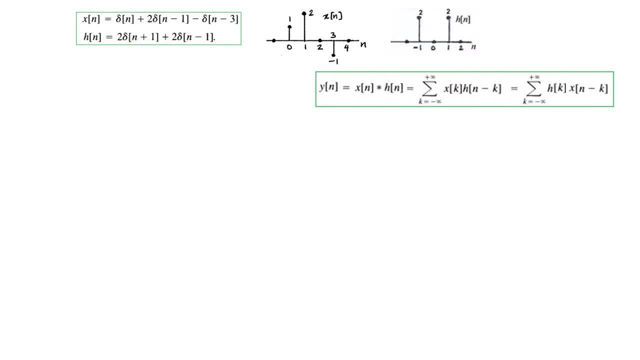 n plus 1. n plus 1 equals 0, means n equals minus 1. so at n minus 1 we plot an impulse of 2, and similarly n minus 1 means we move on the right side. that is, n is equal to plus 1. 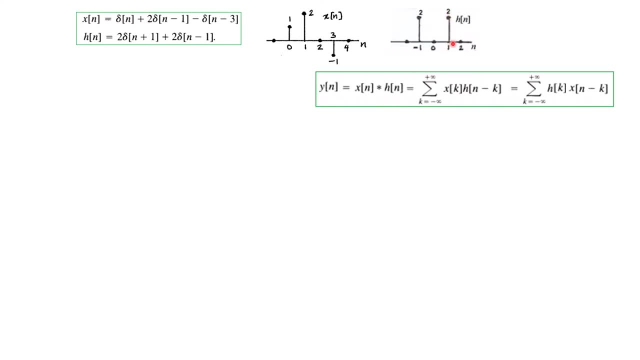 so at plus 1 we again have a impulse of amplitude 2. so this is what is given. this formula we have to keep in mind the formula of convolution yn is xn into hn and it can be written in two forms: sk, hn minus k or hk. 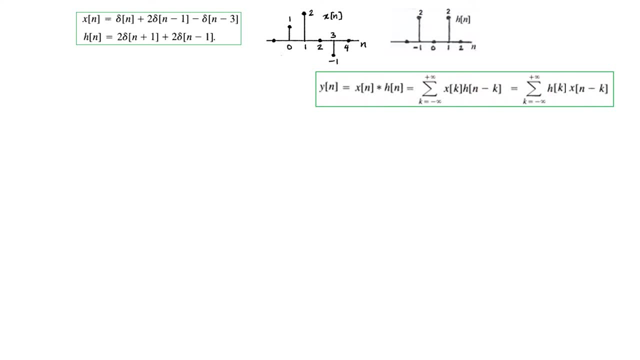 xn minus k, so we can use either of the two, depending on which one is more helpful to us. now let's start the first part. this is what we have to solve, and now, in this case, we are using this formula, the first part, this one, and we are using this because, in this case, xn. 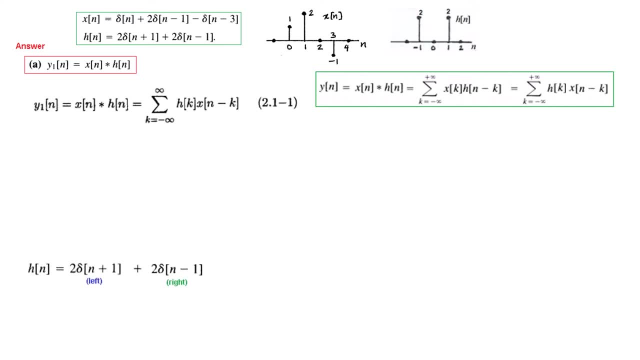 is being moved. so this way, help us more. now, Hn, if you look from here, or even from what is given, I am for my convenience or understanding. I am giving it two names. one is the left part, another is the right part. so this is the left part here and this is the right part here, and so Y1, now this. 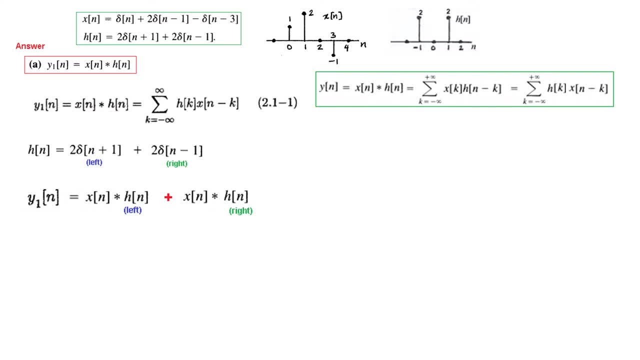 Y1 is Xn convolution Hn. we can write this as Xn convolution Hn left part plus Xn convolution Hn right part, and that means if we put in the value of Hn left and Hn right, it will look like this: Xn convolution 2, delta n plus 1 and similarly the right hand side. now we 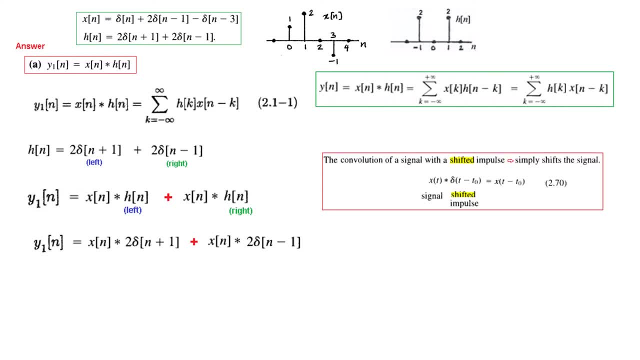 will use a property. That property says that convolution of a signal. so this is signal convolution with a shifted impulse. now this is shifted impulse. the impulse is shifted to point T0. this will imply that simply shift the signal. so the signal Xt is actually shifted by T0. so this: 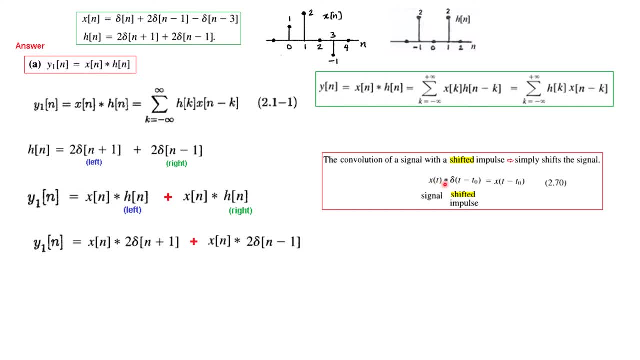 formula will apply here And if you look carefully, they are very similar: Xn- 2 delta n plus 1, and Xn multiplied by 2 delta n minus 1 can now be written as 2 times this 2 X and shifted by n plus 1, so Xn plus. 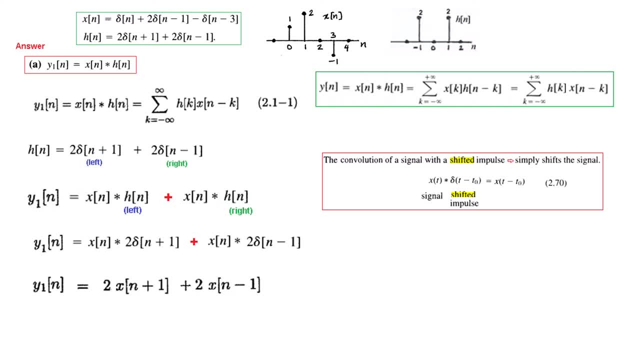 1 and similarly here, 2 times X shifted by n minus 1. so this is the general answer that we have. 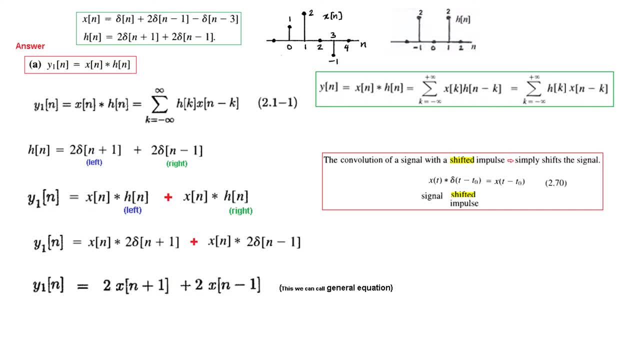 Now, if you need to plot this, then we will have to be a little more specific. so let's see how we do that. 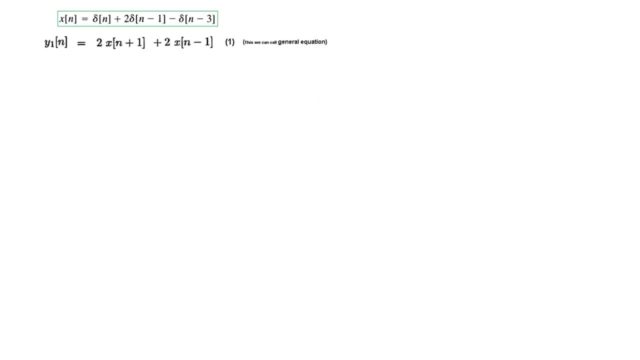 1. this equation 1 can be interpreted as: multiply X2 is equal to 1. Xn by 2, multiply Xn by 2 and replace n by n plus 1, so this is: n has been replaced by. 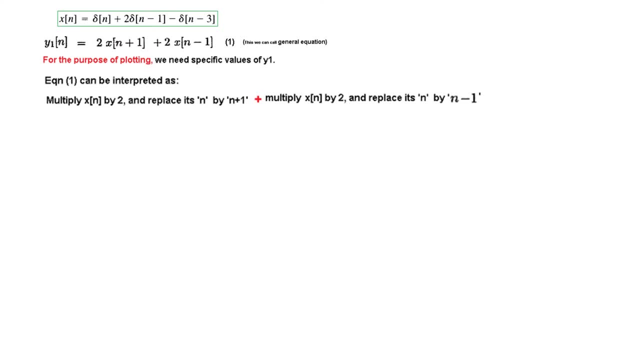 n plus 1. similarly plus sign, multiply by 2 and replace n by n minus 1. so we will use this technique- and this is what is Xn given- to modify Xn. so now look carefully. 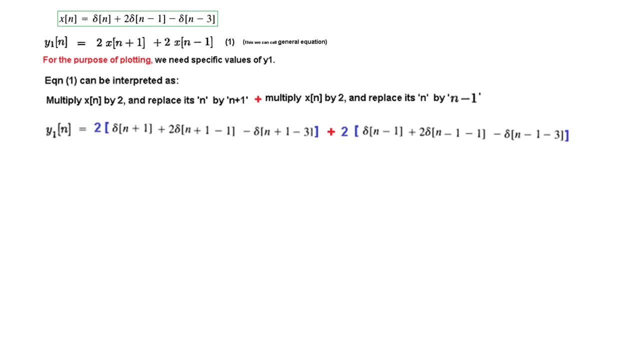 I'm multiplying this whole thing: Xn by the left hand side, so 2 multiply by this whole signal, only shifted by n plus 1. so this n has been shifted by n plus 1. here also n has been shifted by n plus 1, and here also n has been shifted by n plus 1. so this is the left. 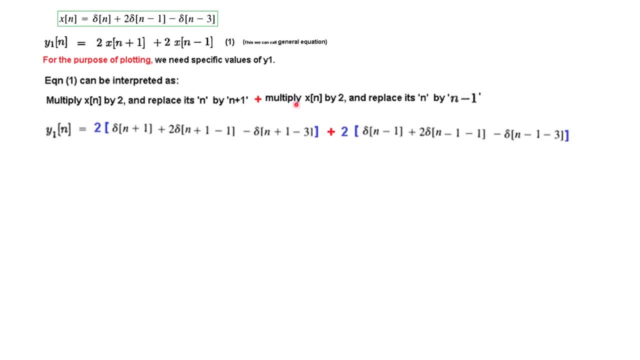 part, this part and the. You have to know here this is the right part- plus again 2 times and shift all the ns by n minus 1. again, this n is shifted by n minus 1. this n is shifted by n minus 1 and similarly. 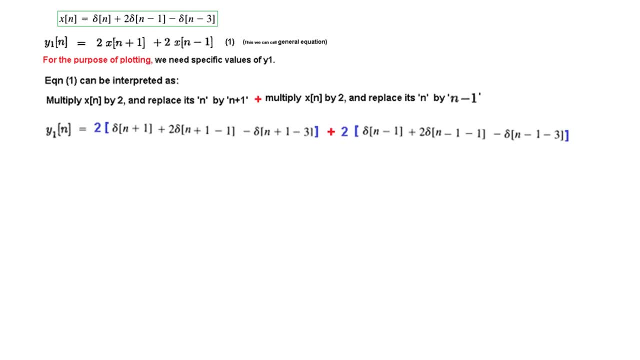 this and now we can simplify. so I hope you can follow these steps here and plus minus 1 will just give it, and so simplifying all this and further adding the like terms, So this will be our final answer for Y1n And now we can easily plot. You can see this. 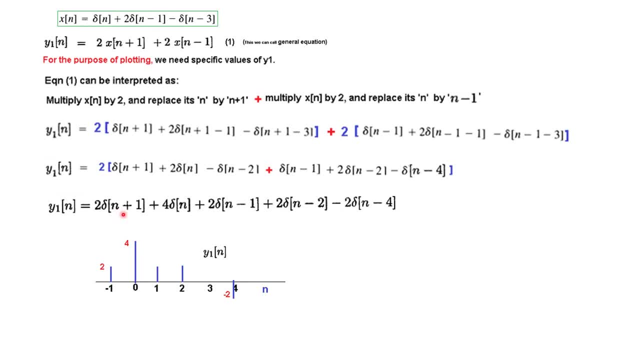 is an amplitude of 2 and located at n plus 1 equals 0, means n equal to minus 1.. So at n is equal to minus 1, we have an amplitude of 2.. Similarly, n is equal to 0, the amplitude 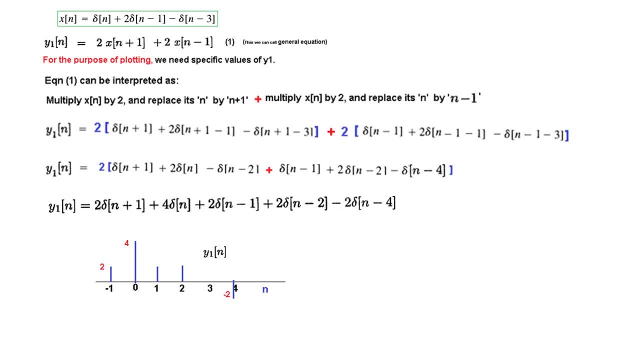 is 4.. And here n is equal to plus 1,, the amplitude is 2.. Here also 2.. At 3, there is nothing, and there is no n minus 3.. So at 3, it will be 0. And here, at n is equal to 4,, it is minus. 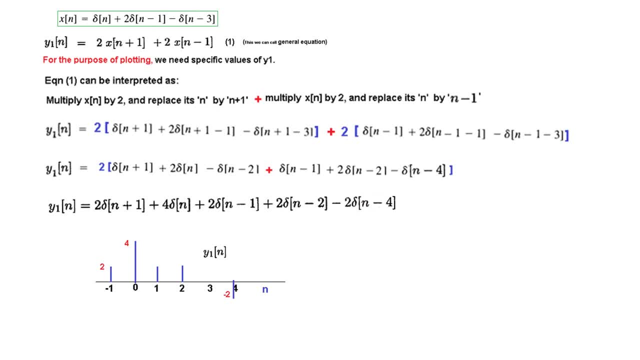 2. So we go in the negative direction. So this is the final plot. Now I will tell you an easy way to verify, or even you can solve, if it is not specified which technique you have to follow. And that easy way is that first of all we write xn. You see this one as an amplitude. 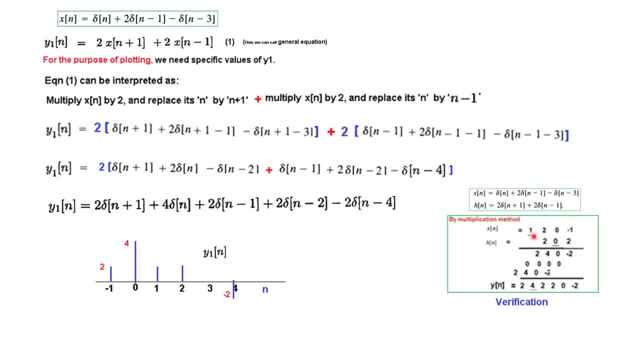 a and it is located at 0. We mark 0 by a dash, Then the amplitude 2.. So we write 2 and it is on the right side of this one. So we write it at the right side. Then there is no amplitude. 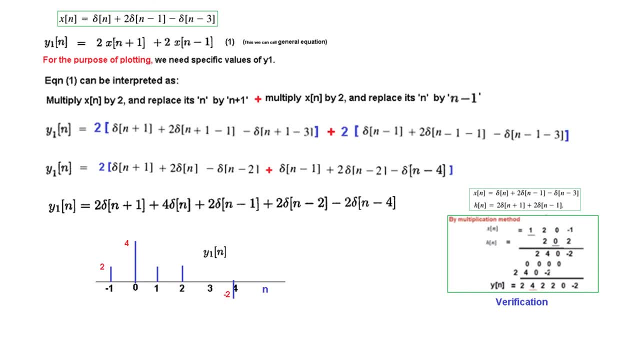 for n minus 2.. So we put it as 0. And then the amplitude for n minus 3 is minus 2.. So we write minus 1.. So we write minus 1.. So this is xn. Similarly, hn is 2 at on the left. 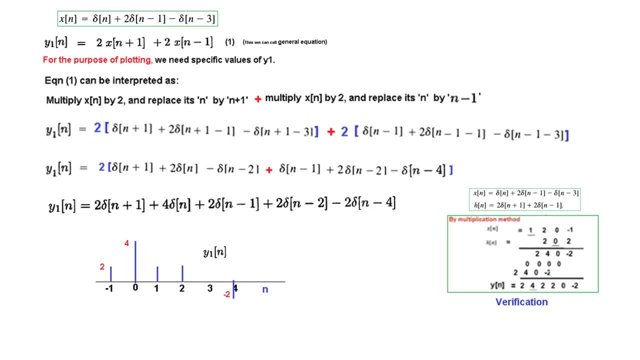 hand side of 0. This is 0. So 2 amplitude. Then there is nothing for 0. So we write it 0. And then on the right hand side we again have an amplitude of 2. Now this will. 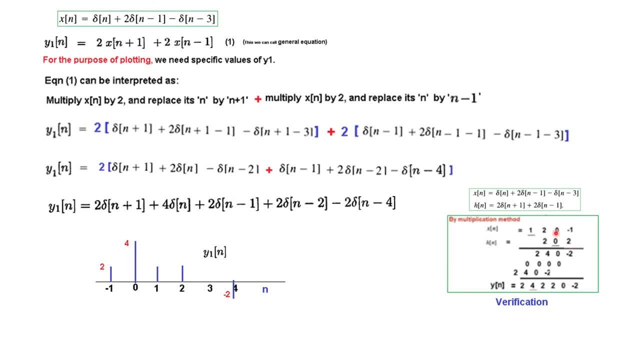 just carry out simple multiplication from right hand side And then addition. So this is the final answer. Now where do we put the 0?? If you look, there is nothing on the left of this 0. And there is only one element on the left. 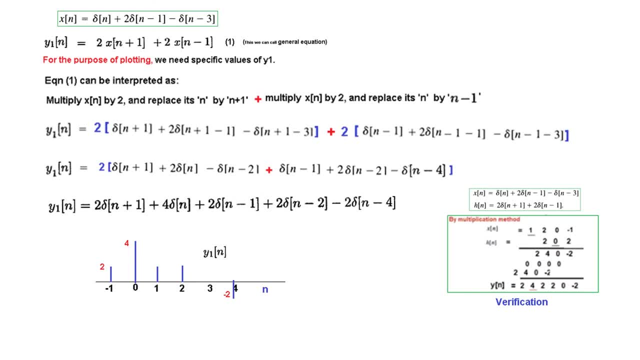 of this, 0.. So total, our 0 is one left of the leftmost, Sorry, one right of the leftmost. So in this case the 0 will be one right of the leftmost. That is, 0 will be here And it is exactly same. You can see amplitude 2, 2.. Then amplitude: 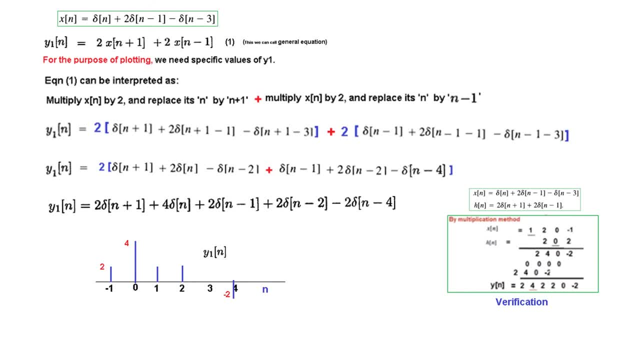 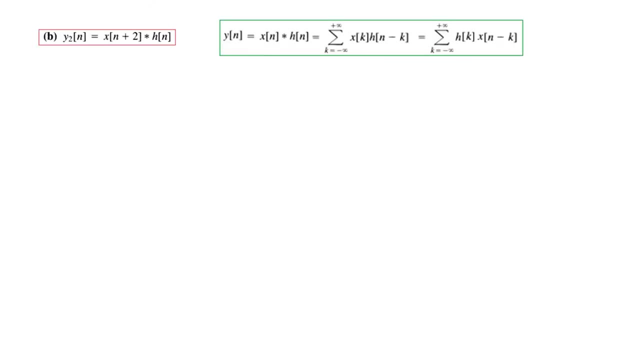 4 at 0. So amplitude 4 at 0. Then 2, 2, 0. So 2, 2, 0. And minus 2.. So this is first part and its verification we did, And now we go to the second part, The second part. 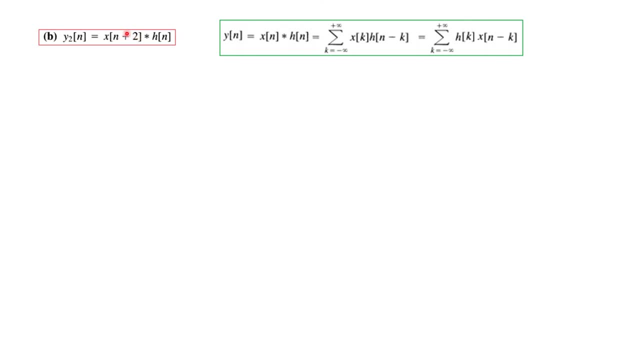 the first part is that in now, in this case, the x n has been shifted by 2. So it has shifted to negative side, And we will again follow this formula Now. here x n has been shifted. Therefore, this one is with x n shifted, So it is logical to use this formula. Okay Now. 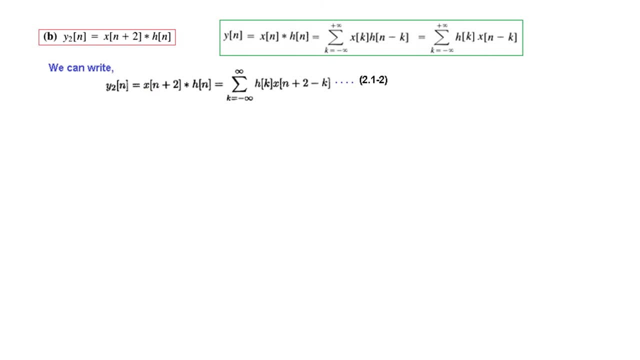 we can write y, 2.. This and the summation. in this formula you can just simply see h k, h k, x, n plus 2.. Now the n has been replaced by n plus 2, because here also in the question, x is now n plus. 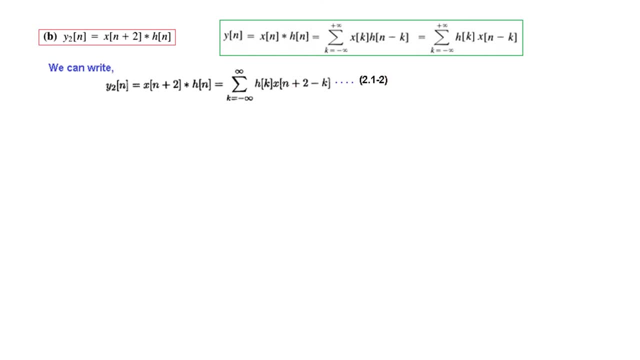 2, remaining remains same, That is minus k. Now, since we have calculated the final value of y 1.. So we haveан plotted it. it is fruitful to relate y 2 with y 1 for further insights. So if you can relate y 2 with y 1, then we exactly knowfrom y 1 how much we have to move. 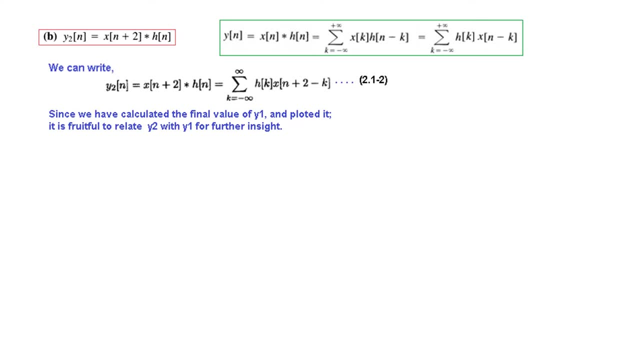 left or right, etcetera. So let us relate it Now, comparing 2 point 1: 2. That means this equation with 2 point 1: 1. That is the original equation for y 1. So this is negative for y 1.. So if you simply put it in the x 1, then 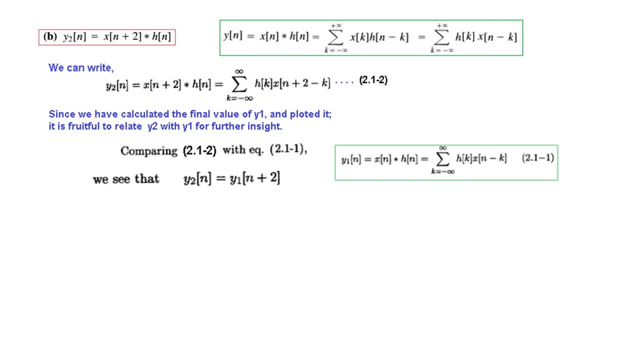 it is true that 2 point 1, 2 is negative for x 1.. Now, this way we can see that now let's is y 1 and this is y 2. if you just compare h k and h k is same, x n plus 2 is in place. 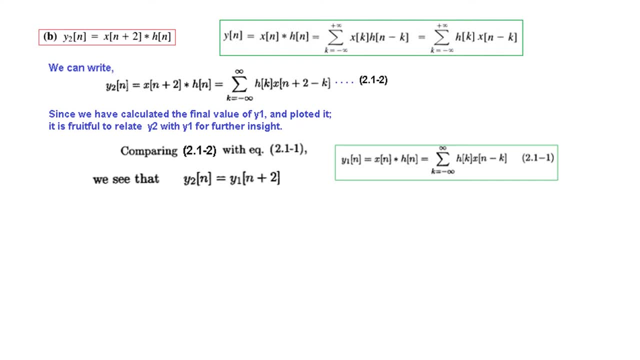 of a n. so n in y 1 has been replaced by n plus 2 and y 2, so we can write that y 2 is nothing but y 1, with n replaced by n plus 2. so this is y 2, and now you can see that. 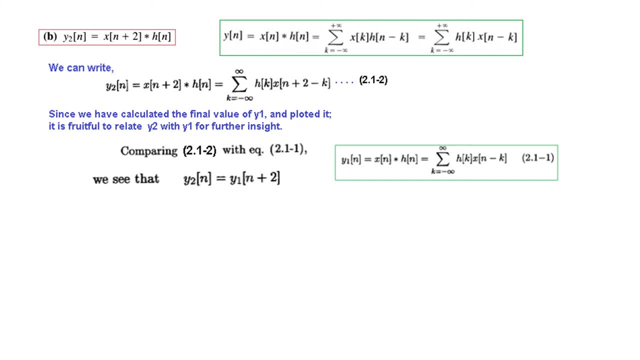 what we have to do. we have to plot y 1 and then shift the whole thing by n minus 2. that is n plus 2, that is on the minus side, on the left hand side, and if you want to go into more details, then now this was y 1.. 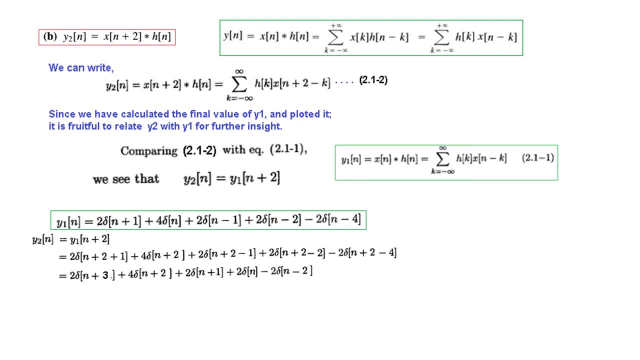 So we shift every n in y 1 by n plus 2. so here we are now writing n plus 2, here we are writing n plus 2, and all the n's are replaced by n plus 2. simplifying. this is the final equation. final. 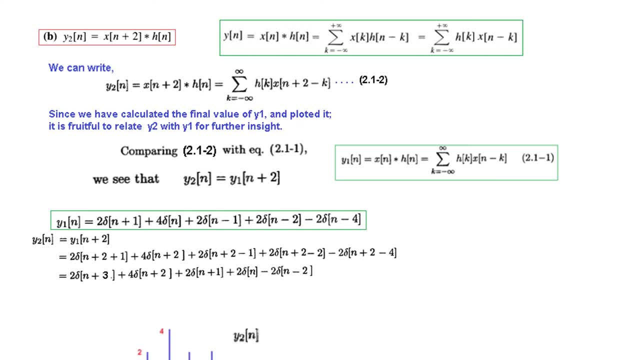 value for y 2 and, as I told you, we can plot from this directly, or this is nothing but y 1 shifted towards left by n plus 2.. So here we are now writing n plus 2 and all the n's are replaced by n plus 2, simplifying. 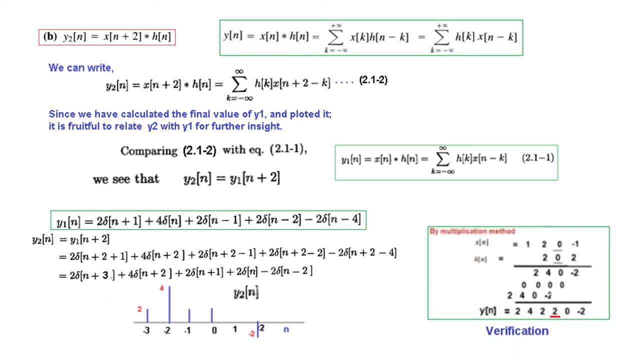 this is the final equation. final equation of algebraic notation'. 0 is the nextimposition of y 1 to y 2. I am writing c January 1000. we will have Modln on next day and hn remains same. we multiply same way. we get this answer. now where do we place? 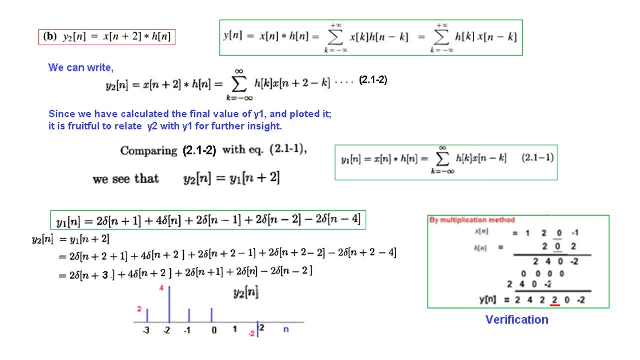 the zero. now, if you look, the left of zero, we have two values here and the left of zero we have one value here. so our zero will be three values to the right, so one, two and three. three values to the right. this value is of zero. and similarly, now you can see- 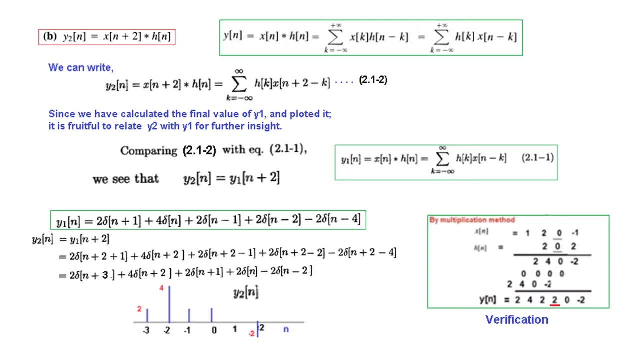 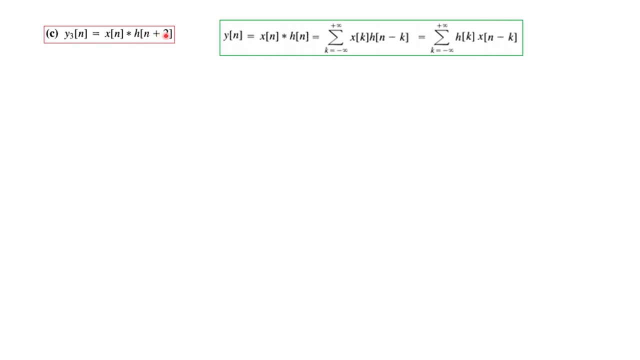 from this graph that our zero is two. on the left of zero is again two and the left is four and further left is two. so we just match with this value. so this is the verification process. we have y3 in this case. now hn has been shifted instead of xn, so we can now. 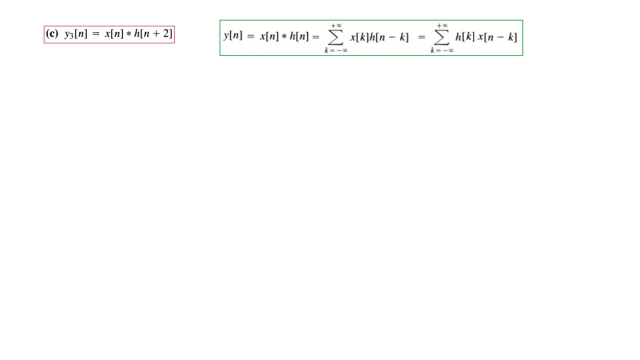 use this function formula. here h n is shifted and we follow exactly same technique. that y 3 is x conversion: h n plus 2, using this formula, we replace n by n plus 2, so this is y 3, we compare. 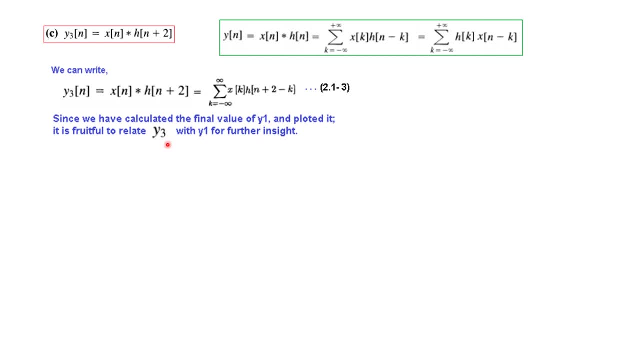 it with again y 1, so this is y 1 and this is y 3, no difference, except that here also n has been replaced by n plus 2, so we can then say that y 3 is nothing but y 1, n shifted. 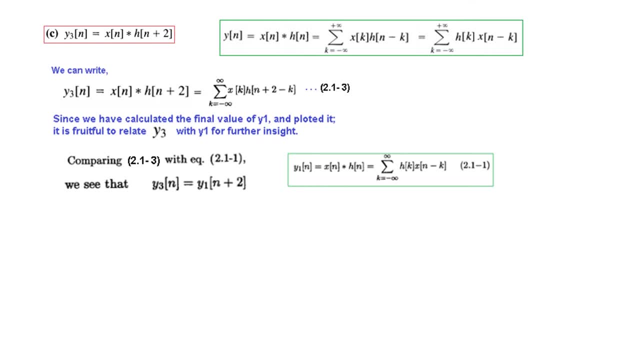 by plus 2,. that means in this case also the whole diagram will move left by 2, so we can say that y 3 is nothing but y 1, and so this was y 1,. we replace all the n's by n plus. 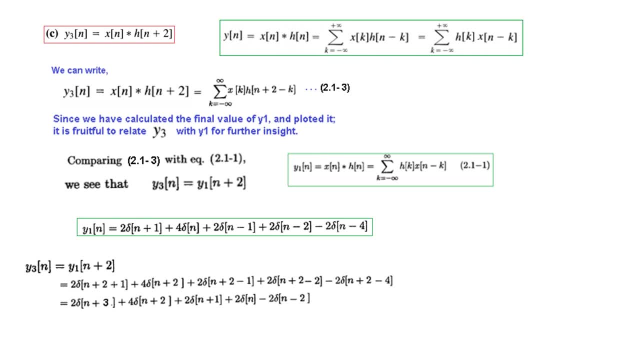 2,. so this is the final answer and you can, I hope, easily plot this. I hope this gives you an understanding how you can solve this type of a problem by mathematical means, not graphical means, through algebraic equations. thank you. 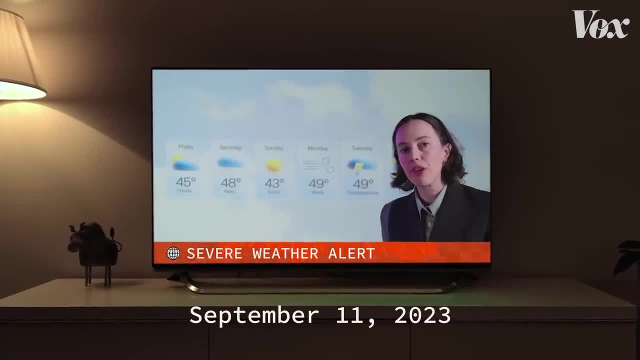 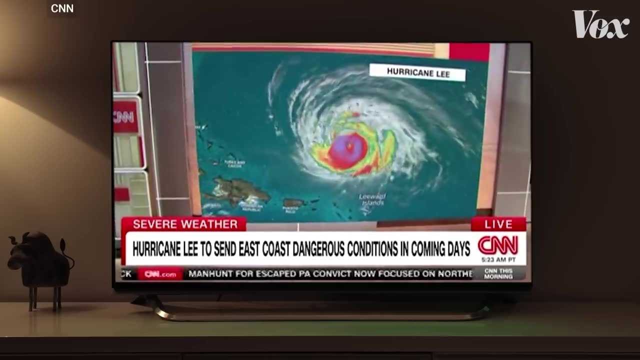 On September 11th 2023, weather predictions in the northeast of the US sounded like this: All eyes are on Hurricane Lee. The storm has strengthened back to a Category 3.. We're expecting it to make a northward turn over the next few days. 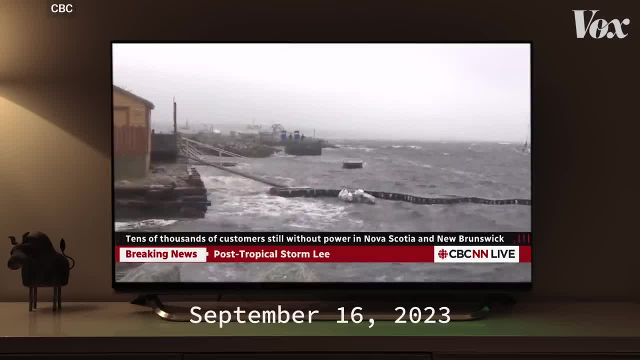 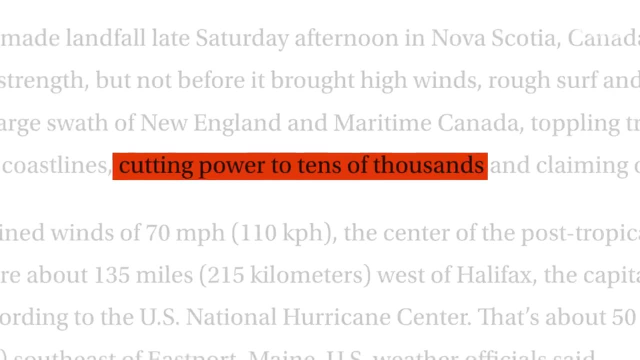 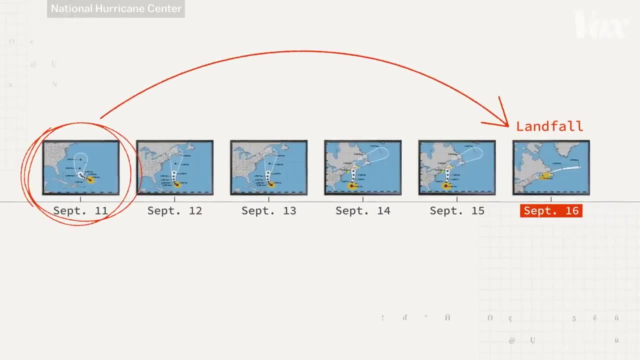 By September 16th, after being downgraded, Storm Lee made landfall in Nova Scotia, Canada, flooding roads, downing trees and cutting out power for tens of thousands of people along the East Coast. At least five days before Hurricane Lee struck land, weather forecasts had roughly predicted its trajectory. 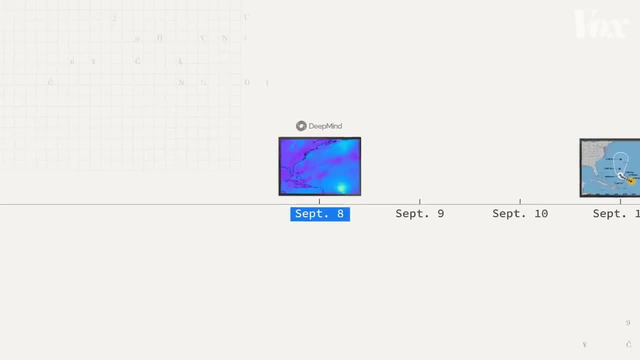 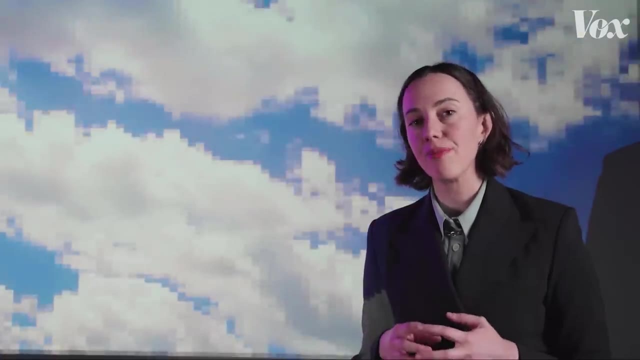 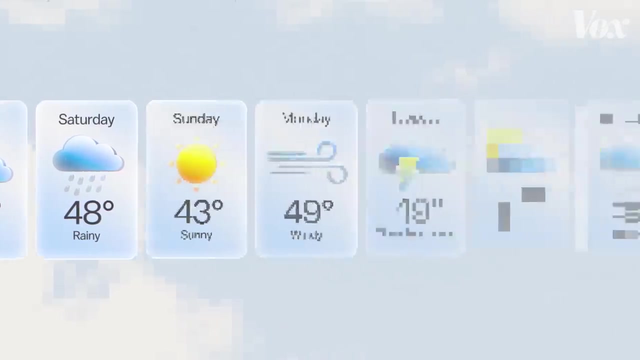 But another forecast beat them. Three days before weather stations, an AI model created by Google predicted the cyclone's path. The AI revolution has reached meteorology, And it's at a time when we are responding to extreme weather more than ever. We're about to find out if it'll help us prepare by bringing the future into clearer view. 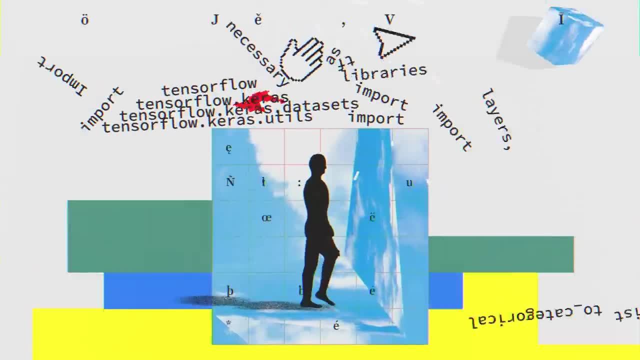 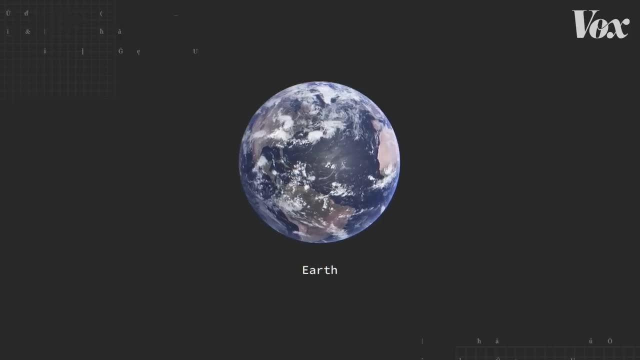 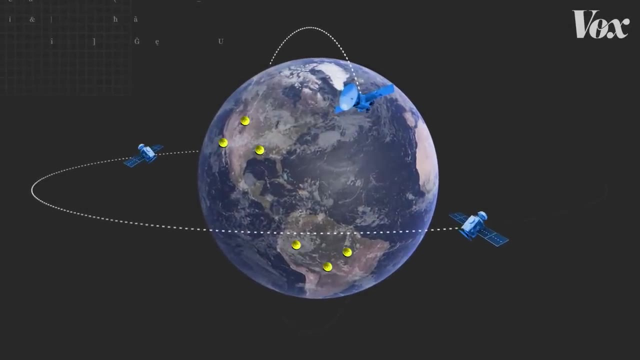 NASA Jet Propulsion Laboratory, California Institute of Technology. Predicting future weather more than a few hours out starts with creating a snapshot of Earth's current atmosphere. Scientists do that by collecting data from sources like satellites and weather stations and buoys located around the world. 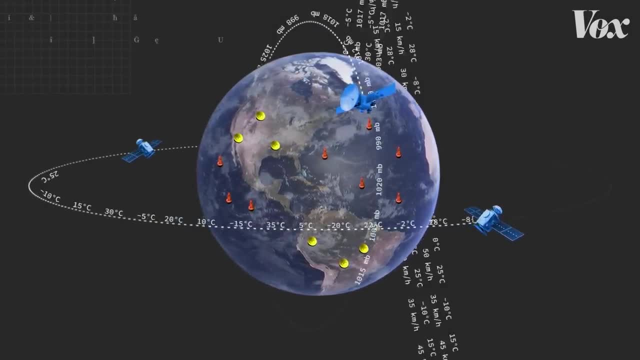 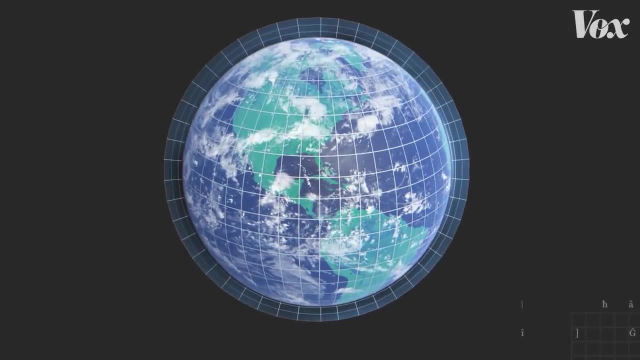 taking pictures of clouds and measuring temperature and pressure and wind speed and humidity. All that disparate data gets fed into computers which generate a three-dimensional map of the Earth's atmosphere. It's a 3D grid of boxes that represent the atmosphere both vertically and horizontally. 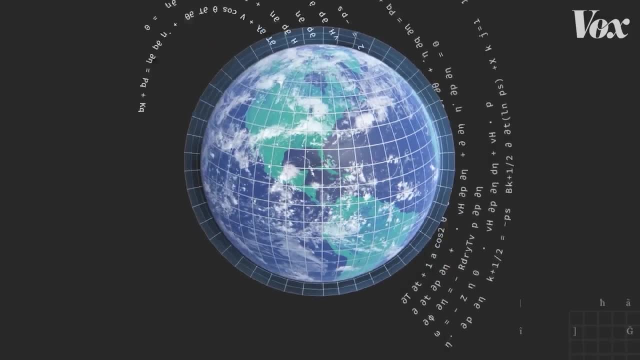 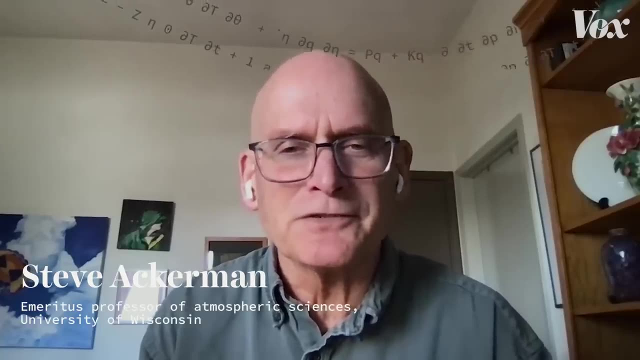 Computers then do a lot of physics to determine how these conditions interact with each other And they produce a forecast. I think any forecast has like 150 trillion calculations. It's pretty amazing. All that math requires some of the world's most powerful supercomputers. 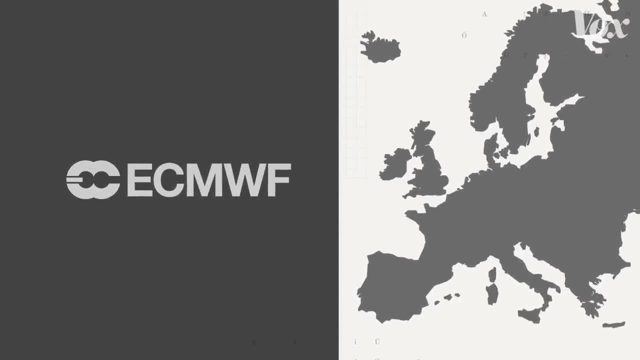 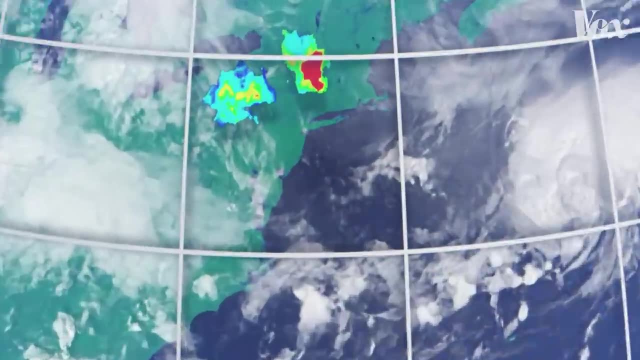 The two big ones are run by the European Center for Medium-Range Weather Forecasts and the National Weather Service in the US To make a local weather forecast from this global map. meteorologists zoom in and refine their own forecast with their local expertise. There's too many gaps in the data we can measure. That means forecasts get blurrier the further out you go, Which is why the big weather centers don't just generate one forecast. They tweak the initial data and produce up to 50 forecasts.